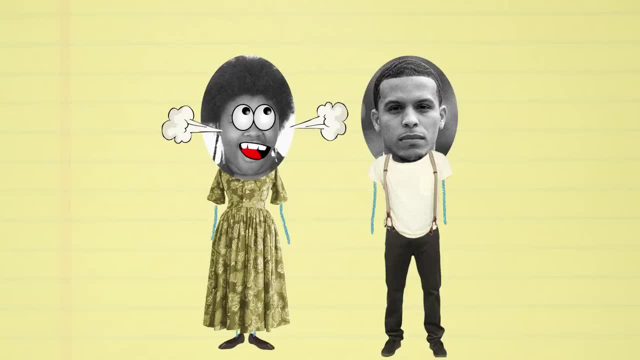 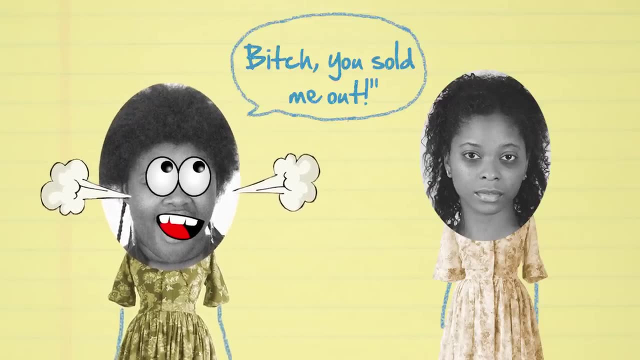 five across da face. But whenever Harpo try to keep her down, Sophia ready to bang out like a real bad bitch. She put Harpo in his place. Sophia real pissed at Celie and ask her why she sold her sister out. Celie just say: she hatin' cuz she wanna ball like Sophia. Later one of Mister's on the side, honey Suge- get sick and Celie gotta look after her long term. At first Suge actin' like a bitch towards Celie, but when she realize how sh** Celie's life be cuz of Mister, she decide she gotta stay and look out for. 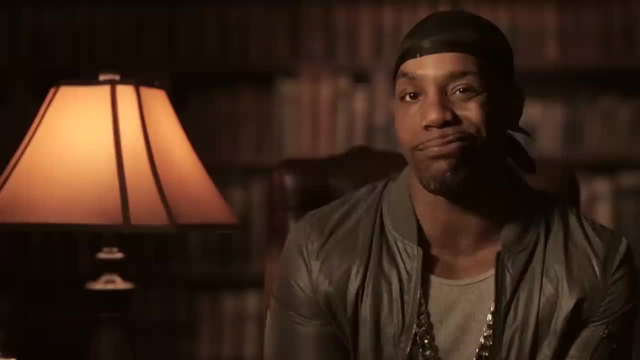 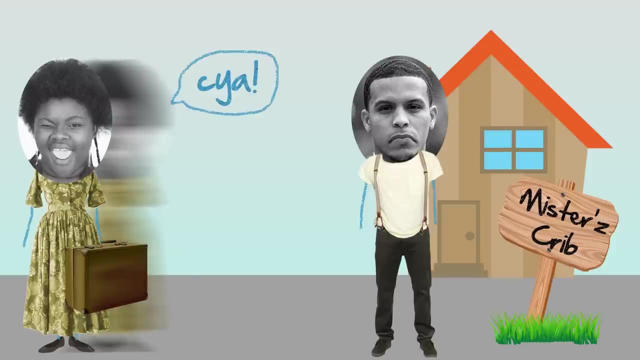 her Meanwhile, Celie can't keep her mind off of Suge's bangin' body. Mm true that Eventually Sophia get tired of Harpo always flexin' and leaves his ass. But when Harpo got some other girl named Squeak, Sophia come back and pop her right in the mouth WORLD. 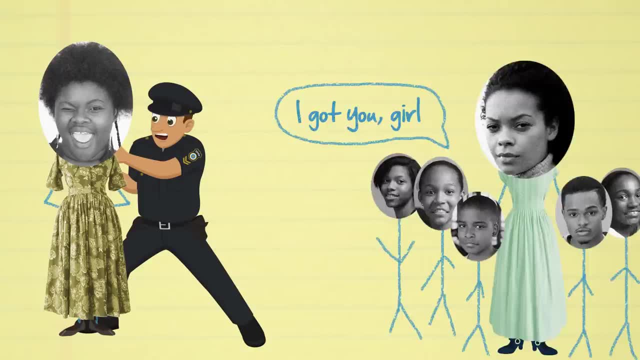 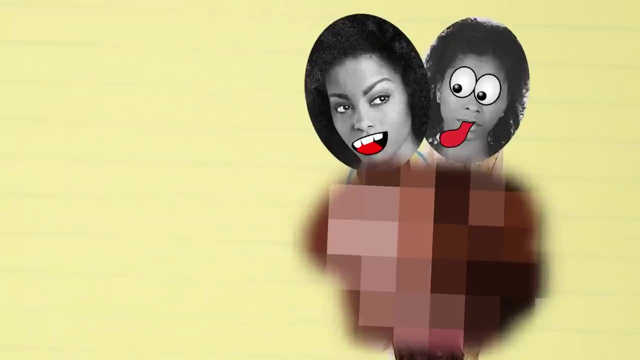 STAR. But after Sophia gets in trouble with da law, Squeak start lookin after her kids and they become cool Suge, leave for a while and come back with some scrub husband, But dat don't stop her from gettin' freak nasty with Celie. Now this is literature. 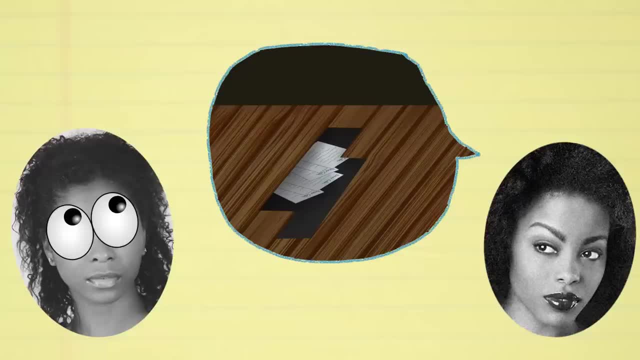 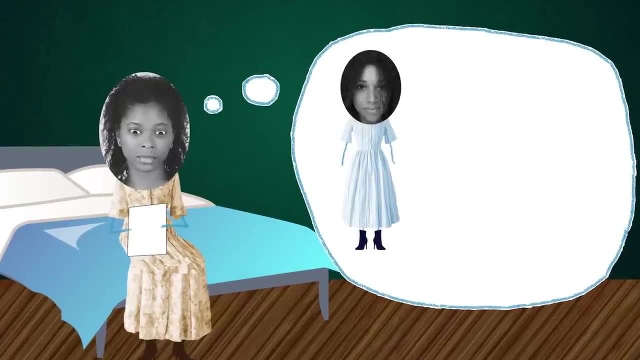 When Celie start talkin about how much she miss Nettie Suge say she been seein some letters. Miss da been stashin This punk-ass been withholdin Nettie's letters to Celie, Dem letters sayin dat Nettie hooked up with two missionaries named Samuel and Corinne and they been spreadin. 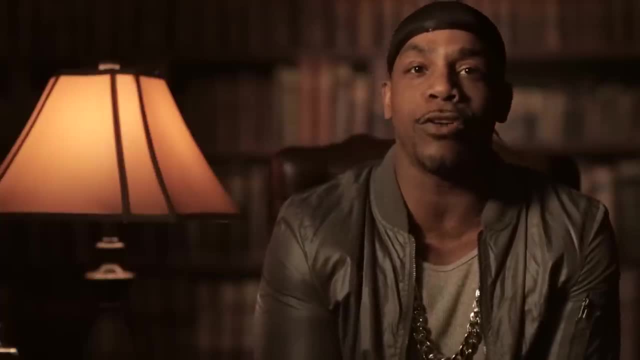 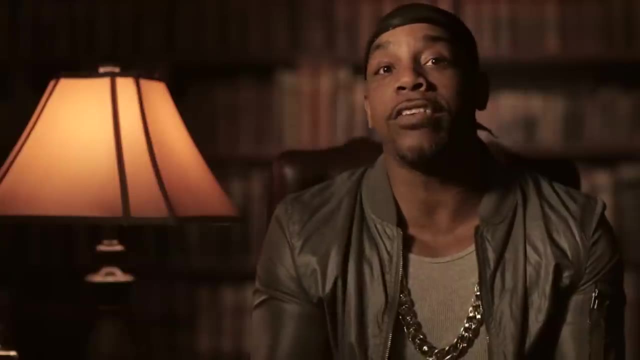 the good word in Africa. Not only that, but apparently Alfonso didn't kill Celie's two kids, Naw, they were adopted by Samuel and Corinne back in the day. Ain't dat some sh**? Also turns out, Alfonso ain't even her real daddy. Finally, tired of Mister's. 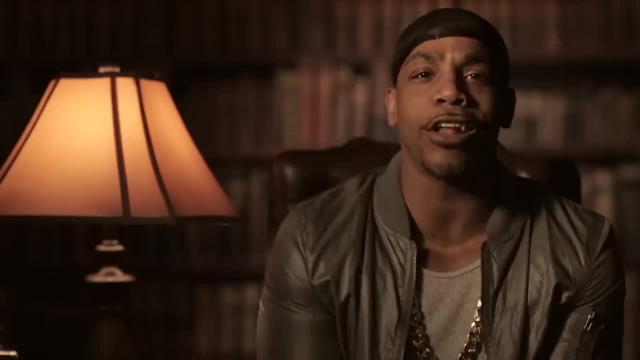 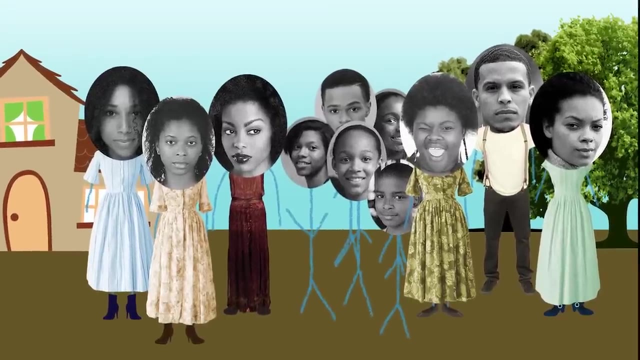 bullsh**. Celie Squeak and Suge bookin to Tennessee to start a new life. When Alfonso up and dies, Celie be like. Celie inherits da whole family house After 30 years of bein apart da whole family. 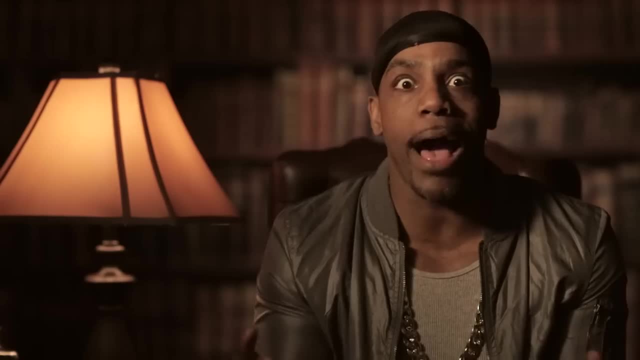 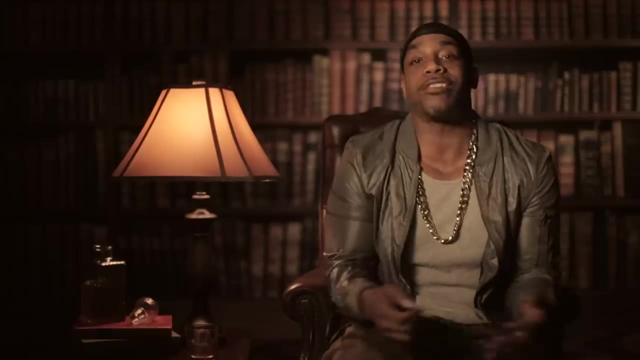 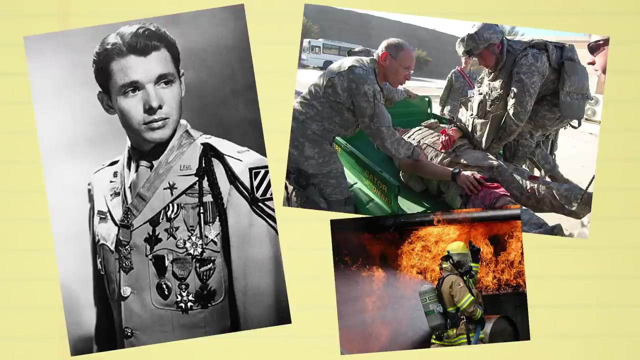 includin Suge, come together in da old house where it all started. Bout damn time somethin good happen in this book. Sh** Most historical novels always jivin about men doin real trill. sh** conquerin turf, winnin wars, sacrificin they selves. But with the color perp my girl. 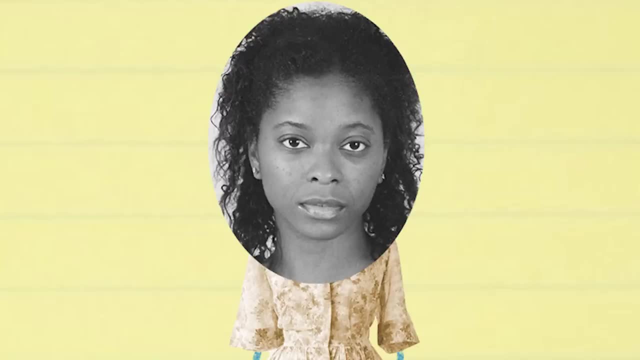 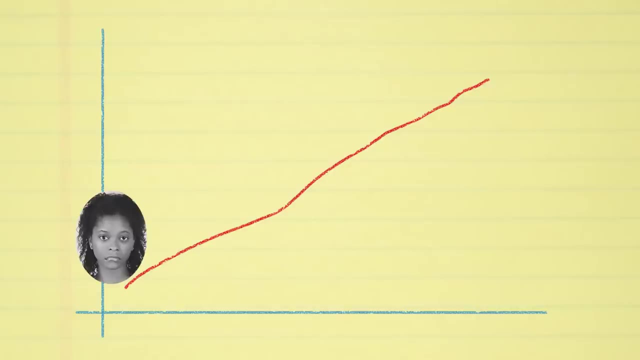 AWOC, flippin dat sh** upside down, showin a woman beastin through oppression And eventually overcomin da same men who, deez old-school books, deem heroic. Dem bustas might keep Celie down at first, but by da end she come out a strong, independent woman doin her thing.